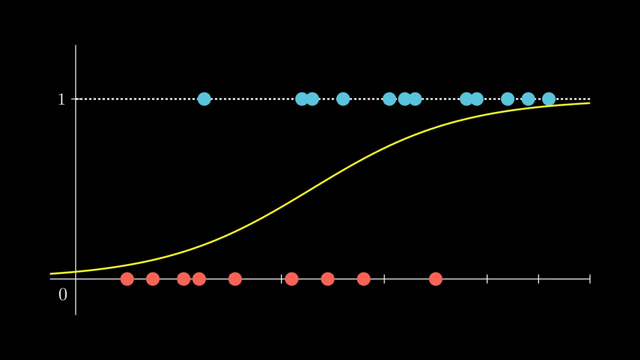 value respectively. You then fit this S-shaped curve called the logistic function to this data. It can then be used to make predictions of probability, whether or not an event will happen, such as: given so many hours of rain, what is the probability of a flood Notice? 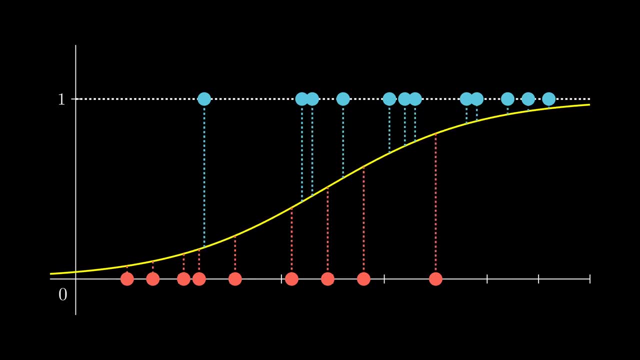 how that these points can project themselves onto the logistic function and we can use maximum likelihood estimation to fit the curve, which we'll talk about shortly. Notice that there are these middle points where there is a mix of true and false cases. If these 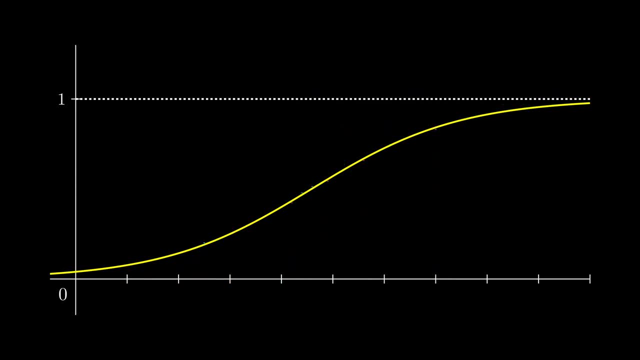 points follow a transitional trend of increasingly showing an event more likely to happen or not happen. you will see that that S-shaped curve will climb or decrease respectively. We can then leverage it to predict probability between 0 and 1.. Let's take a case where we 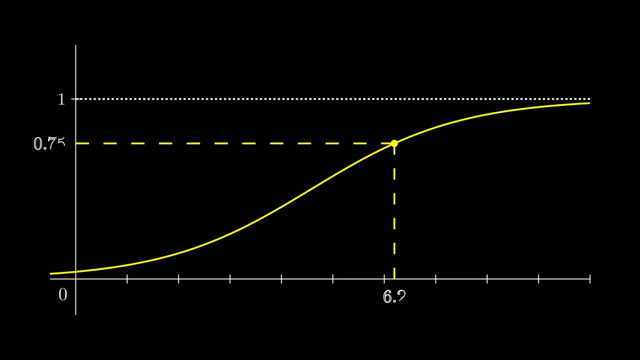 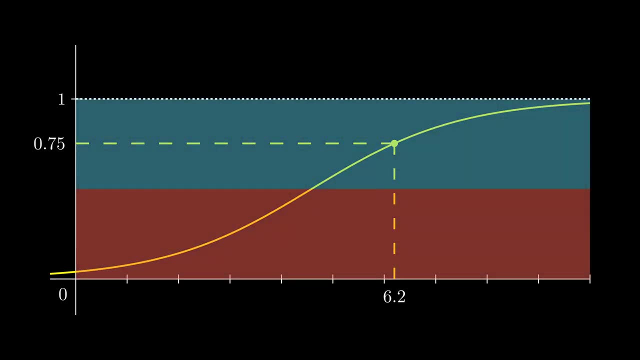 expect 6.2 inches of rain and this is going to result in a 0.75% probability of a flood. If we define a threshold- say 0.5, and anything greater than 0.5 will be true, anything less. 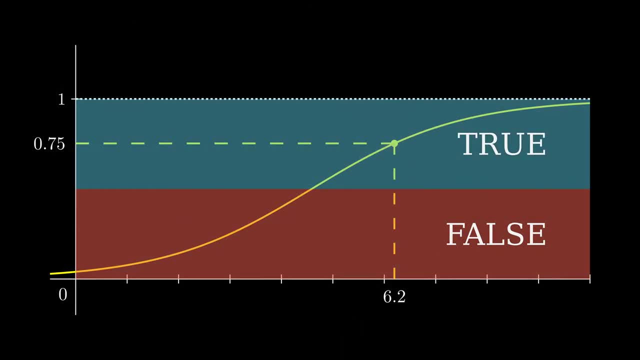 than 0.5 will be false. we will then predict there will be a flood. We can move this threshold based on our needs. For example, if we set it to 0.8,, this would actually categorize as false and there won't be a flood. We can also reduce it to say 0.2, and set a much. 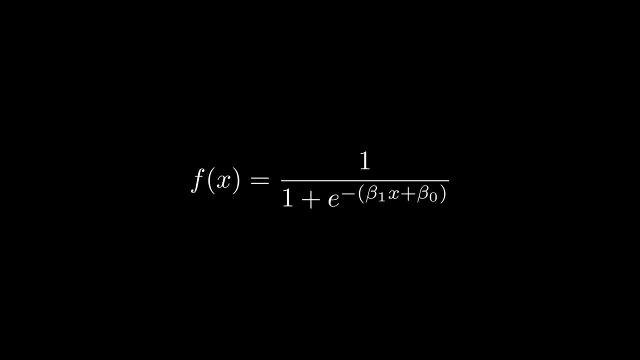 lower barrier to classifying a flood. This is the function that produces that s-shaped curve. E is Euler's number, which is a special constant, That beta 1x plus beta 0 is a linear function. That is actually the log odds function. That is: 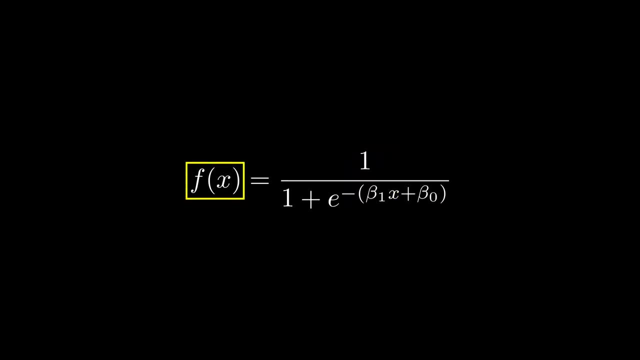 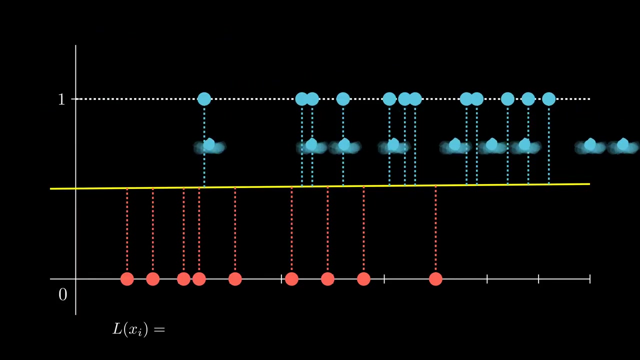 something we will talk about in another video. What's important to know is that this function will produce that s-shaped curve. we need to make predictions. We can also extend this to more input variables to create multi-dimensional logistic regressions, as shown here. Let's talk briefly about maximum likelihood estimation- The way it works. 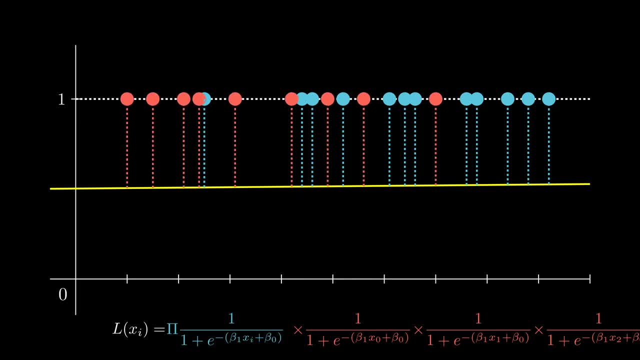 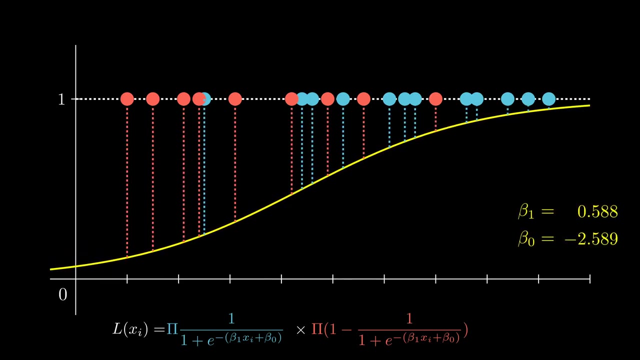 is that we are going to take each of these points, multiply their corresponding likelihoods together and that is going to produce our total likelihood. We need to find the beta coefficients that will maximize the likelihood of our s-shaped curve producing all of these points. This can 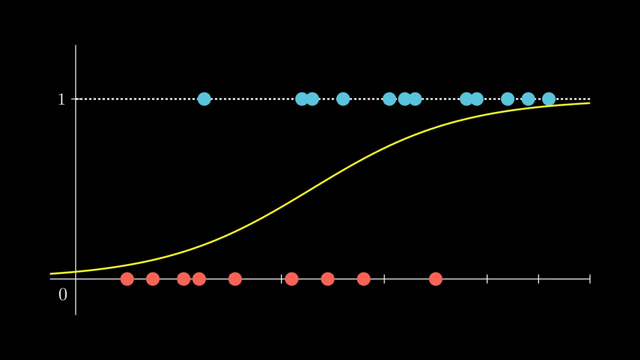 value respectively. You then fit this S-shaped curve called the logistic function to this data. It can then be used to make predictions of probability, whether or not an event will happen, such as: given so many hours of rain, what is the probability of a flood Notice? 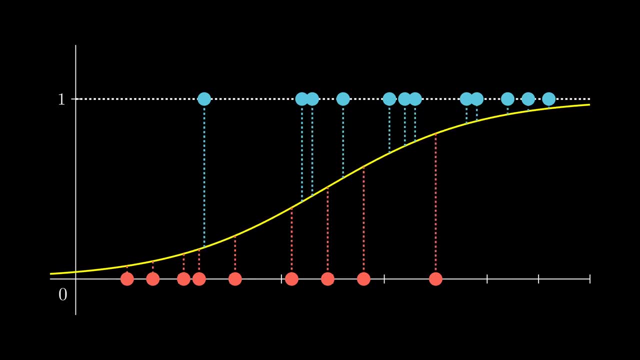 how that these points can project themselves onto the logistic function and we can use maximum likelihood estimation to fit the curve, which we'll talk about shortly. Notice that there are these middle points where there is a mix of true and false cases. If these 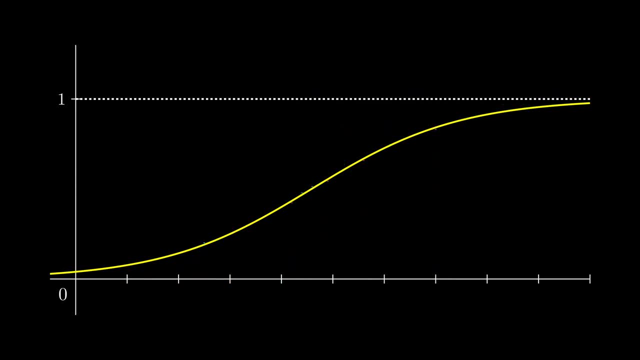 points follow a transitional trend of increasingly showing an event more likely to happen or not happen. you will see that that S-shaped curve will climb or decrease respectively. We can then leverage it to predict probability between 0 and 1.. Let's take a case where we 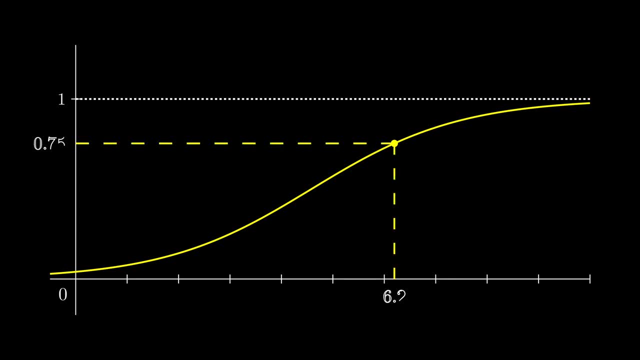 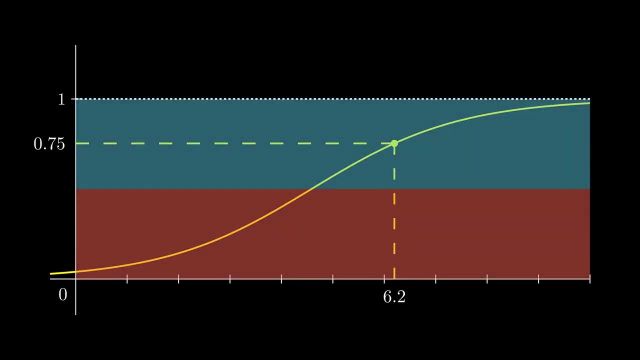 expect 6.2 inches of rain and this is going to result in a 0.75, or 75% probability of a flood. If we define a threshold- say 0.5,, and anything greater than 0.5 will be true. 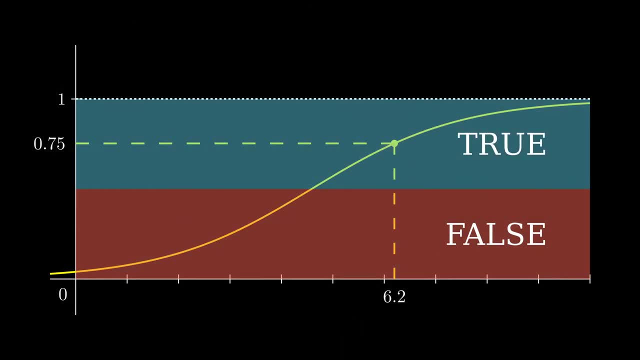 anything less than 0.5 will be false. we will then predict there will be a flood. We can move this threshold based on our needs. For example, if we set it to 0.8, this would actually categorize as false and there won't be a flood. We can also reduce it to say 0.2 and set. 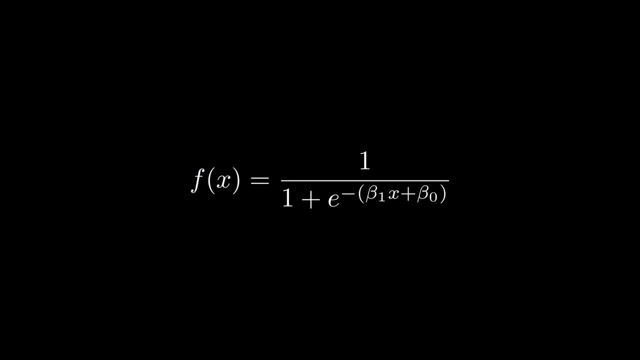 much lower barrier to classifying a flood. This is the function that produces that s-shaped curve. E is Euler's number, which is a special constant, That beta 1x plus beta 0 is a linear function. That is actually the log odds function. That is something we will talk about in another video. 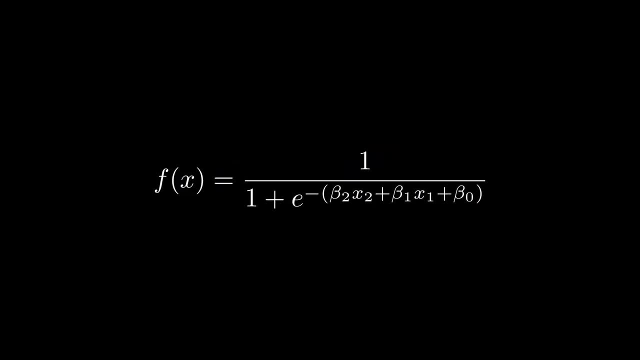 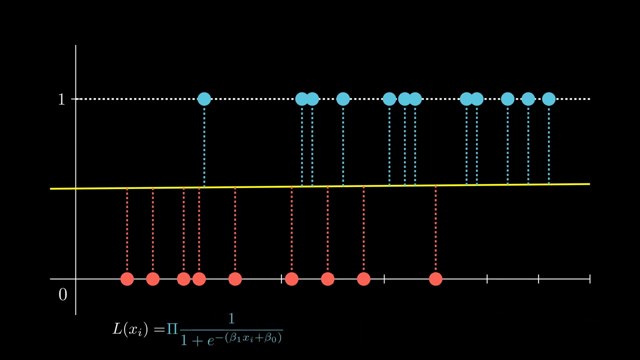 What's important to know is that this function will produce that s-shaped curve. we need to make predictions. We can also extend this to more input variables to create multi-dimensional logistic regressions, as shown here. Let's talk briefly about maximum likelihood estimation. The way it works is that we are going. 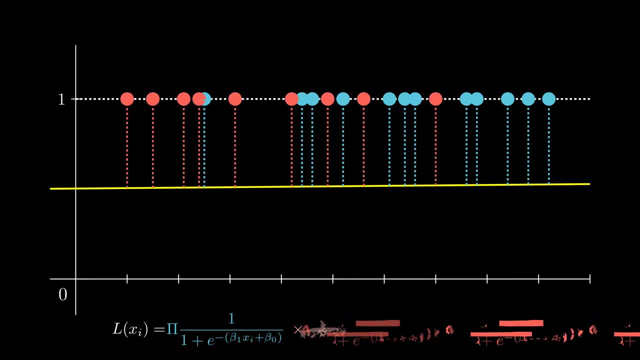 to take each of these points, multiply their corresponding likelihoods together and that is going to produce our total likelihood. We need to find the beta coefficients that will maximize the likelihood of our s-shaped curve producing all of these points. This can be done with gradient.